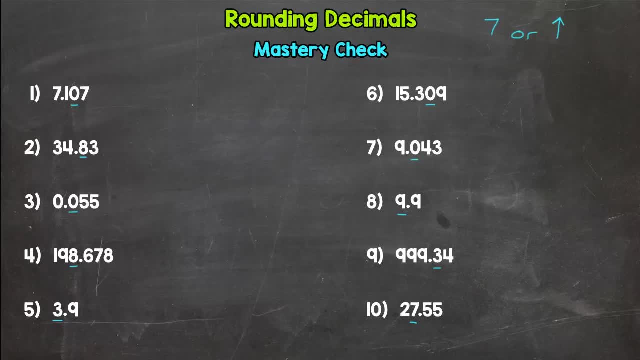 And that will show you have mastery. So when you're ready to go, go ahead and press pause. Alright, welcome back. I'm assuming you have numbers 1 through 10 done, So we're just going to go through the answers and see how you do. 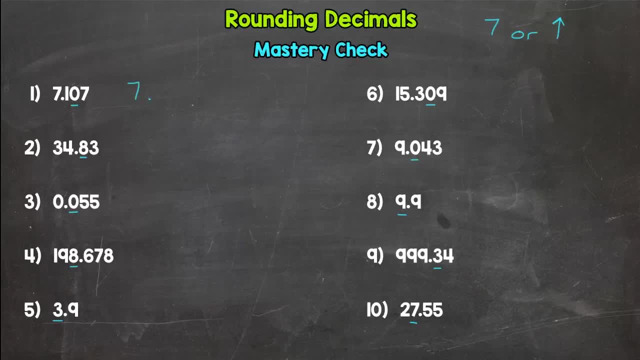 So, number 1, we're rounding to the hundredths place. You should have 7 and 11 hundredths. Number 2, we are rounding to the tenths place. You should have 34 and eight tenths. Number 3, tenths place. 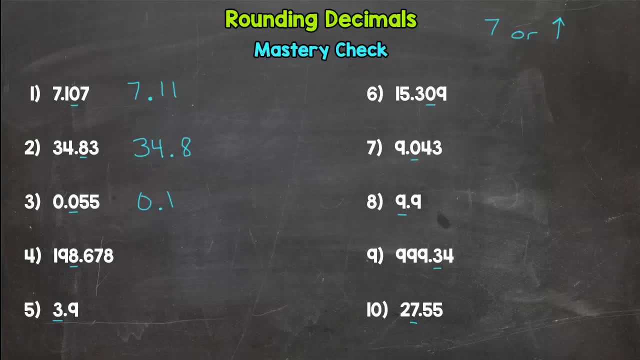 You should have one tenth, Number 4, we are rounding to the nearest whole number or the ones place, And you should have 199.. For number 5, we are rounding to the nearest whole number as well. so you're asking yourself: is that number closer to three, or are we? 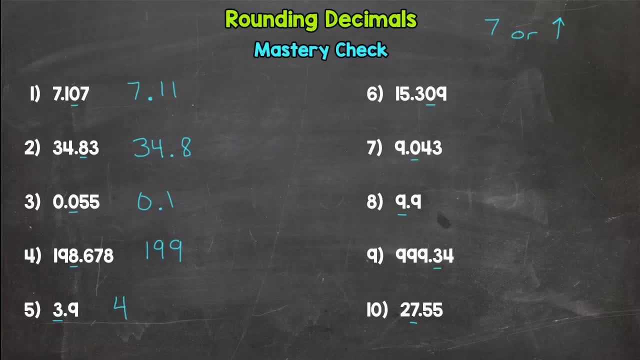 closer to four and that nine tells us we are closer to four number six hundredths place. we should have 15 and 31 hundredths number seven, rounding to the tenths place, and that says stay the same. so if you put nine and zero tenths, 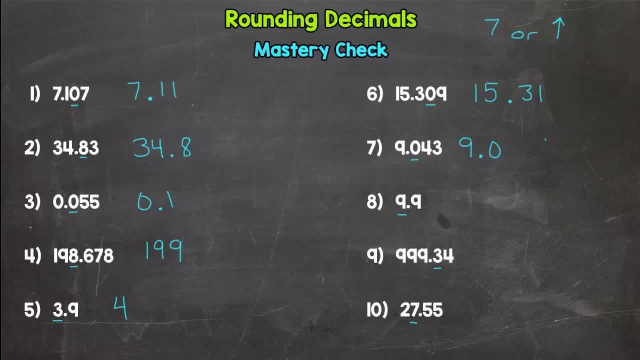 that would be fine, right, but it's just a whole number, so you can just have nine, two these are equal, so it doesn't matter number eight, nearest whole numbers, or so are we closer to nine or closer to ten? this nine tells us we round up to. 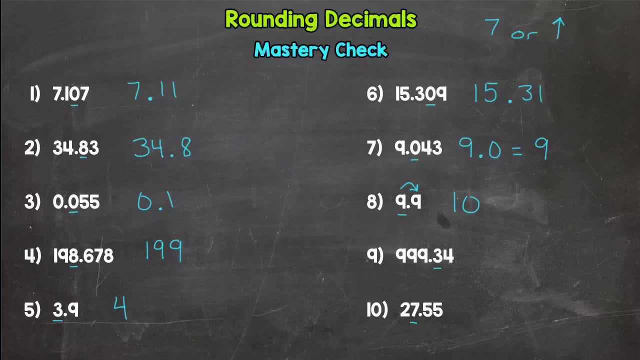 ten, number nine, the tenths place- we should have 999 and 3 tenths, And then lastly, number 10, rounding to the nearest whole number. So are we closer to 28 or 27?? And that 5 in the tenths place says we should round.